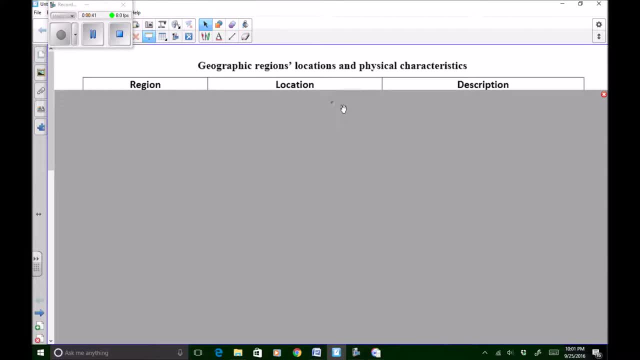 of each region, what the land is like there. And here we go. We're going to start off with the coastal plain. You remember the coastal plain from last year in fourth grade. Well, this year in fifth grade, there's also the coastal plain of not just Virginia, which is included in the coastal plain, but 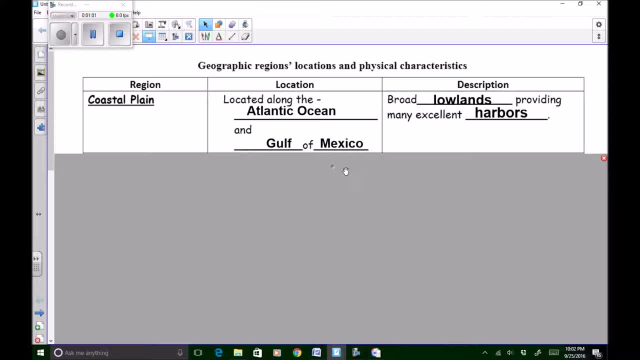 the coastal plain of the whole North American continent. Okay, the location of the coastal plain is located along the Atlantic Ocean and the Gulf of Mexico. The Gulf of Mexico is a large body of water, that is, it borders Mexico to the east and it borders the United States to the south. So, located along the Atlantic, 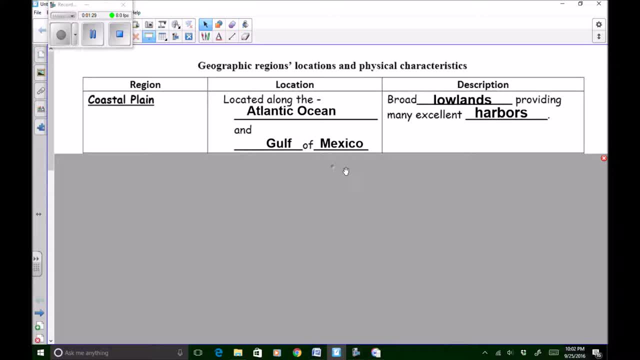 Ocean and the Gulf of Mexico. If you were to describe it, you would describe it as having lowlands that are broad- Broad is another word for wide Broad lowlands- providing many excellent harbors. A harbor is a body of water that is kind of enclosed a little bit by land. 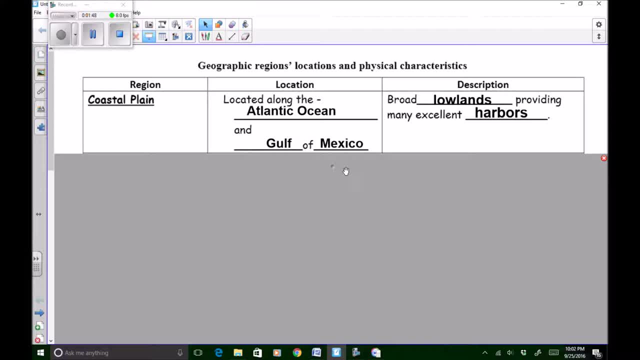 and the harbors are used for importing and exporting goods, such as things from China, things from different countries, and also sending things out of the country to other countries to sell and and as well as people. Okay, so it's a coastal plain located along the Atlantic. 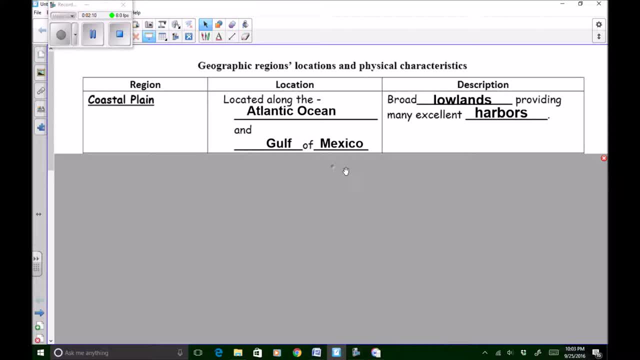 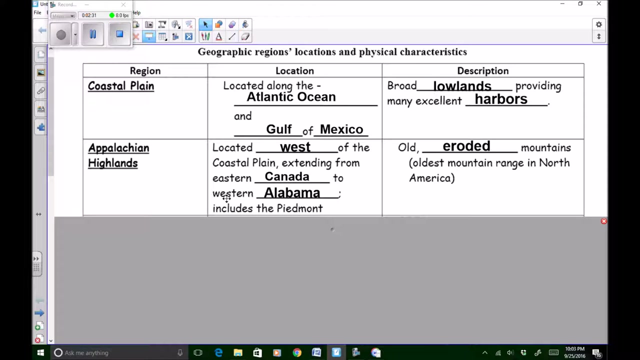 Ocean and the Gulf of Mexico. It's described as being broad lowlands. The land is low there and providing many excellent harbors. The next geographic region of North America is the Appalachian Highlands. The Appalachian Highlands is located west of the coastal plain extending from 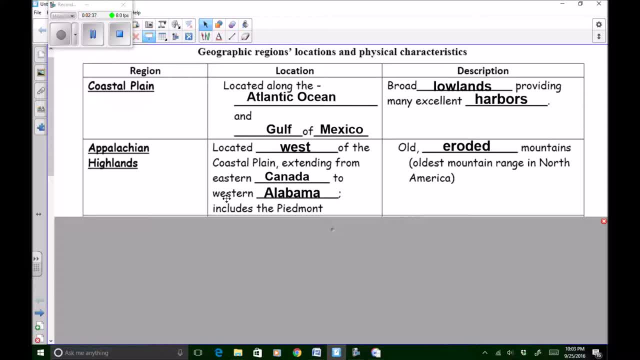 eastern Canada to western Alabama and includes the Piedmont. Okay, so this is the Appalachian Highlands. This is a region that basically includes the Appalachian Mountains, which, of course, are run through Virginia, but it's located west of the coastal plain extending from eastern Canada. the eastern part of 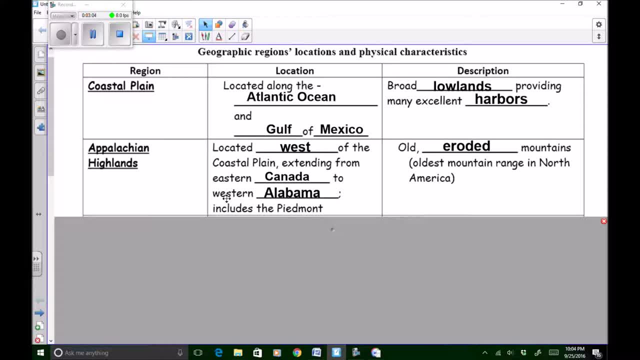 Canada, which borders the United States to the north, our northern neighbor, to western Alabama, the state of Alabama, and includes the Piedmont. To describe this area, you would say it has old, eroded mountains. It is the oldest mountain range in North America. We know they're old because they are eroded. Okay, when we 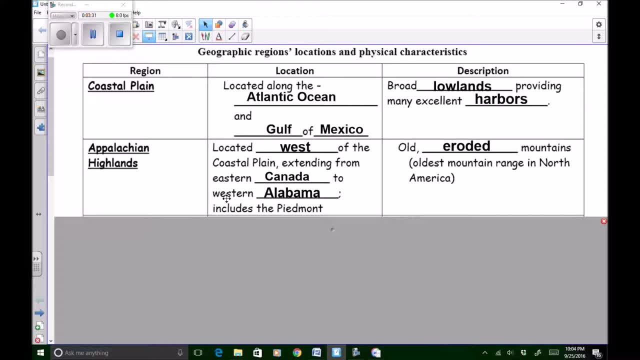 get down and talk about the Rocky Mountains. I'll mention how the Rocky Mountains are steep and pointy mountains, where the Appalachian Highlands and Appalachian Mountains in the Appalachian Highlands are old and rounded and it's because of the erosion. Okay, if you need to pause this video of 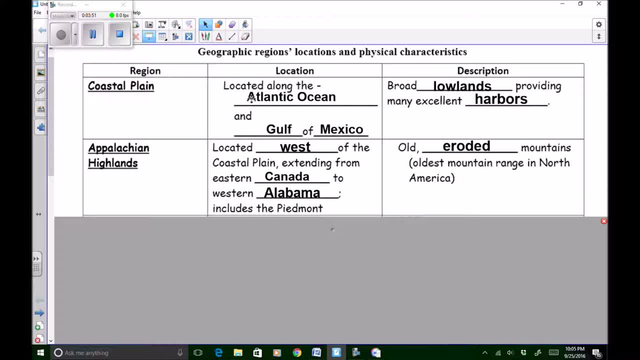 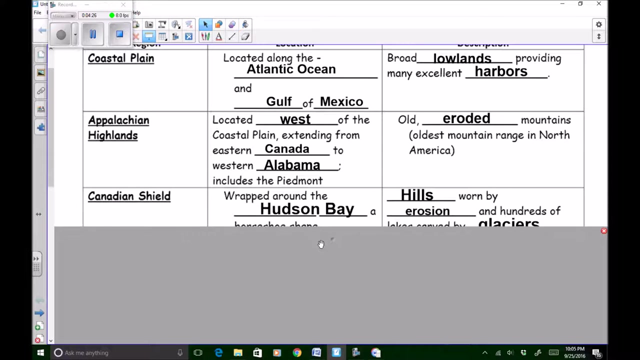 course you can, to catch up, to fill in your blanks here. We'll see you next time. Okay, remember, you can pause this if you need to. I want to go ahead and scroll down so we can get our next region of North America, and that next region is called the. 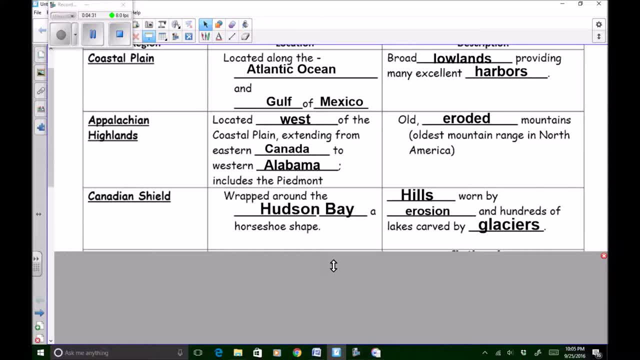 Canadian Shield- The Canadian Shield Now, the location of the Canadian Shield is basically near the Hudson Bay. Hudson Bay is a bay that is close to New York and Canada. It's wrapped around the Hudson Bay, actually in a horseshoe shape. Okay, so the Canadian Shield wrapped around the Hudson Bay in a 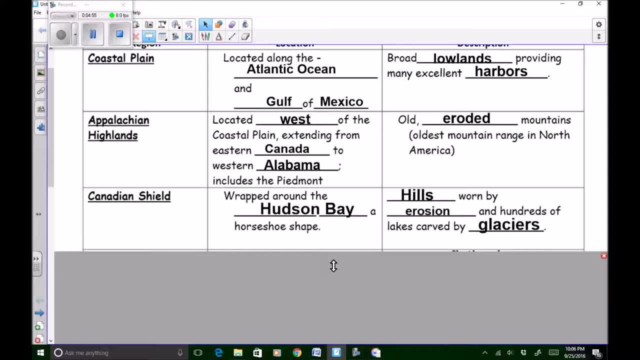 horseshoe shape and if you described the land there, you would say it has hills worn by again erosion. Water has changed and shaped our land so much over the thousands of years that our world's been in existence and the hills of the 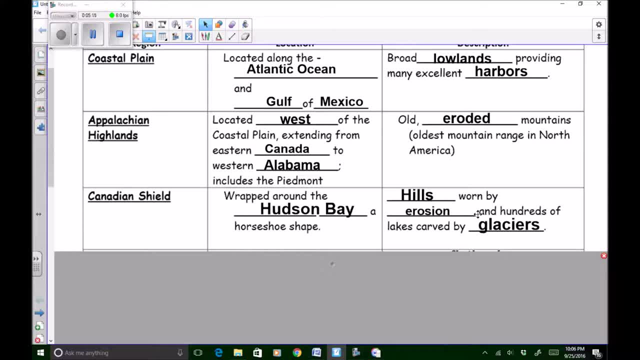 Canadian Shield shield- are worn by erosion and hundreds of glaciers- sorry, not hundreds of glaciers- hundreds of lakes carved by glaciers. all right, that's the Canadian shield. I'm going to scroll up a little bit. remember, of course you can pause and rewind this video if you need to, and we'll go ahead and scroll up to get our 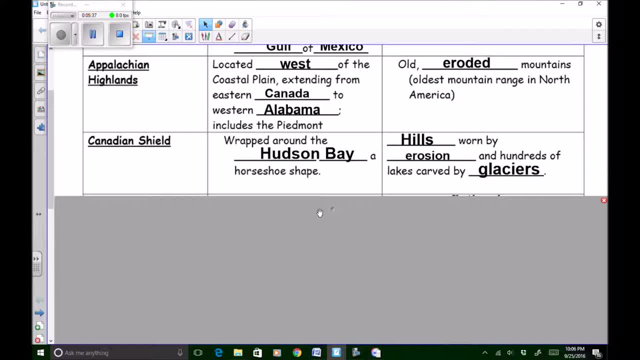 next geographic region of North America, which is our fourth one, is the interior lowlands, is what it's called. they're called the interior lowlands. well, low lands kind of describes it. anyway, it's low land, low in elevation. interior means inside. okay, it's located west of the Appalachian Mountains and east of the. 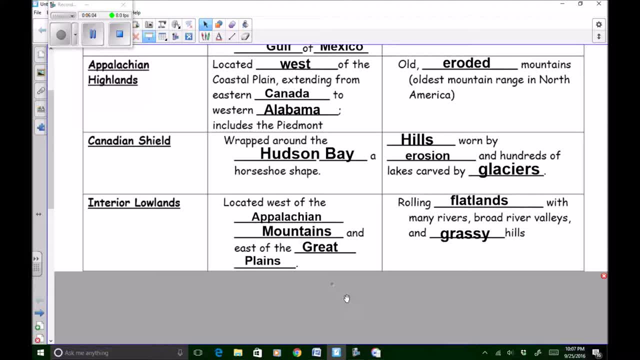 Great Plains now being well-known for the fact that the Appalachian Mountains are located in the west of the Appalachian Mountains and east of the Great Plains. it's kind of in the middle of those two areas. okay, it can be described as having land that is rolling, flat lands with many rivers, broad river valleys and grassy hills. 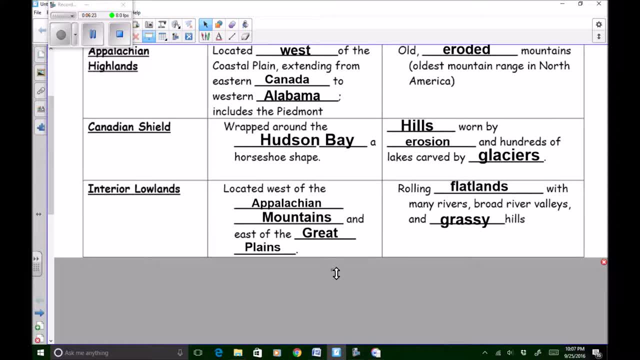 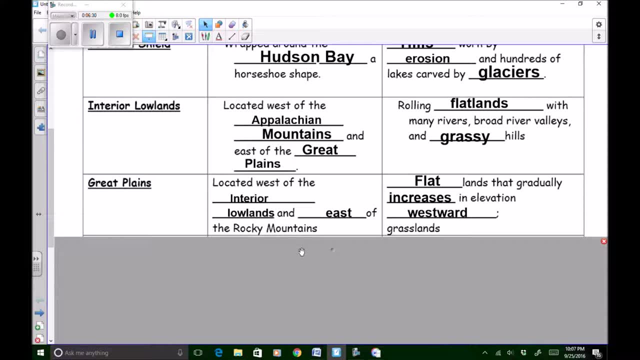 that's the interior lowlands. our next region is the Great Plains. now, the Great Plains is also known as our breadbasket. we call it our bread basket because in the United States that's where a lot of wheat is grown, and when people grow wheat, they harvest it and and they grind it up to make flour. 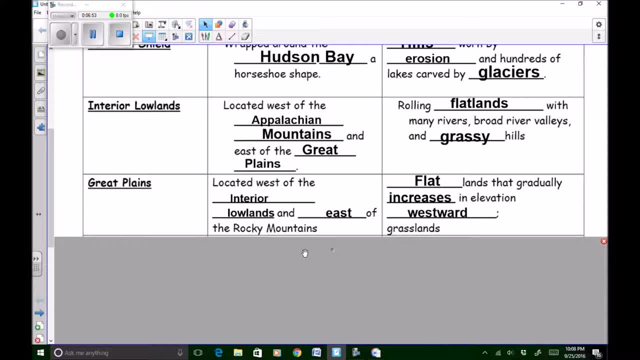 and of course we use flour to make bread. so the Great Plains is located west of the interior lowlands and east of the Rocky Mountains. East of the Rocky Mountains the land in this area is considered to be flat lands that gradually increase in elevation. gradually increase in elevation meaning: 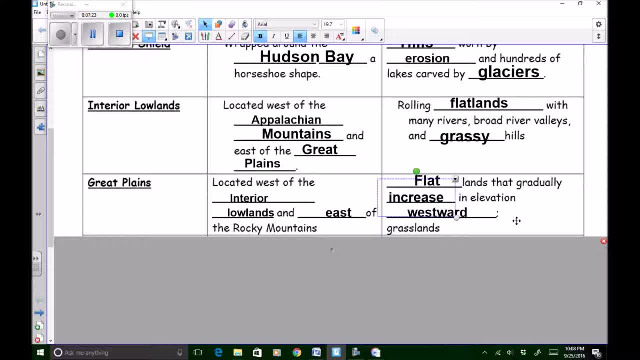 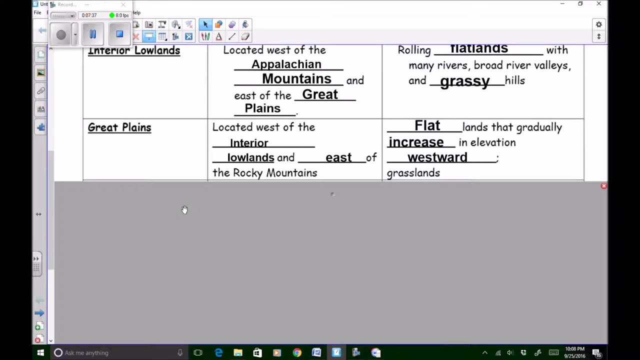 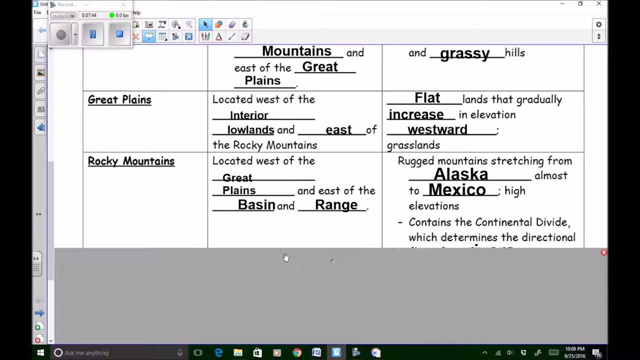 that the further you go west, the higher the land gets. increases in elevation as you go westward and it's coarse grasslands. the Great Plains is a lot of grasslands, a lot of farmland there. all right, our next region. have to scroll this down quite a bit. 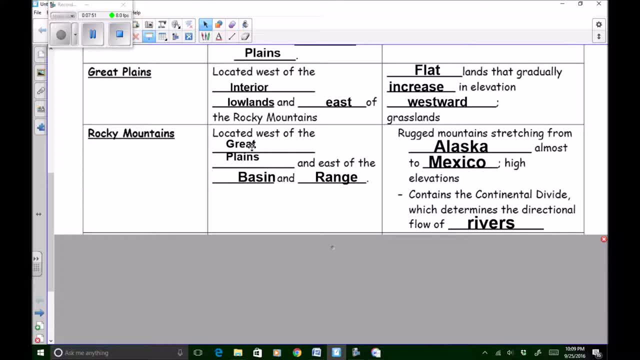 remember, you can pause this if you need to to catch up. the next region is the Rocky Mountains. the Rocky Mountains: if you go to the Rocky Mountains, you're gonna see some ski resorts. you're going to see tall, tall mountains, pointy mountains, not like the mountains around here that are round and covered with. 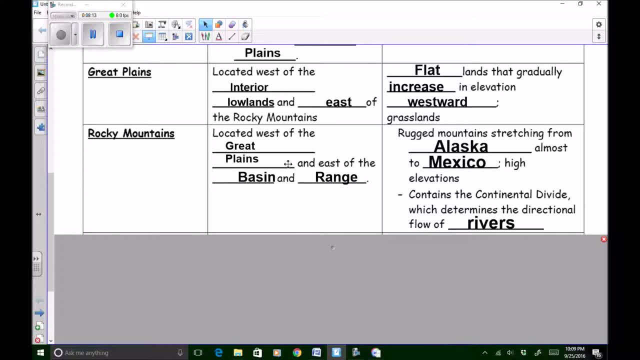 trees, these, these are just rocky, tall, rocky and pointy. they're pretty young compared to the mountains we have here. they're located west of the Great Plains and east of a region called the basin and range- now the word basin. well, if you, when you go to the 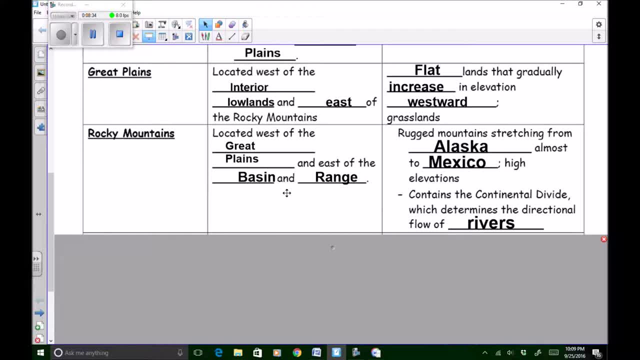 sink to wash your hand in the restroom. the sink part, the bottom part that catches the water. that's called the basin. so imagine a bowl, the basin and the word range refers to. the word range refers to mountain ranges. okay, so the Rocky Mountains, again located west of the Great Plains and east of the basin. 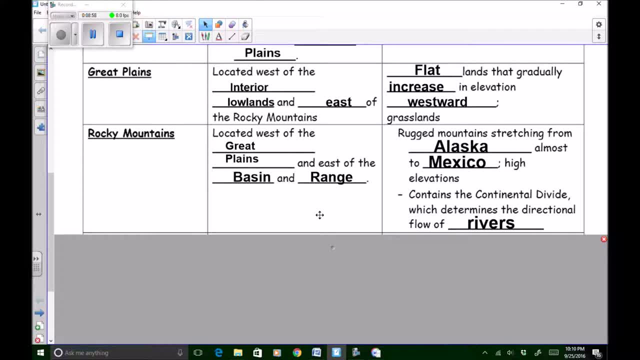 and range. now, if you were described, if you describe this region of North America you would say has rugged mountains stretching from Alaska almost down to Mexico. high elevations, the mountains in Virginia where you and I live, the mountains in Virginia, the highest mountain is five thousand two. 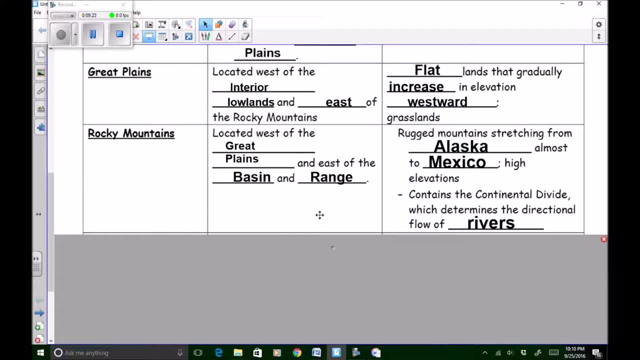 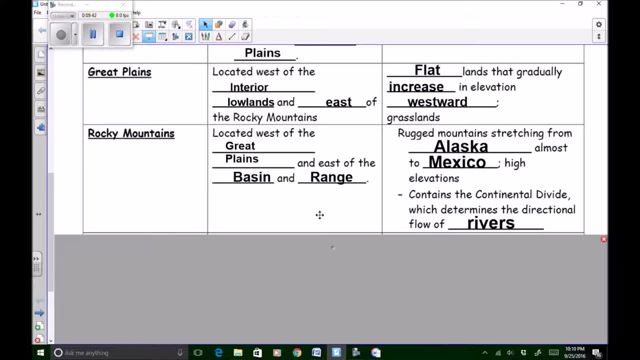 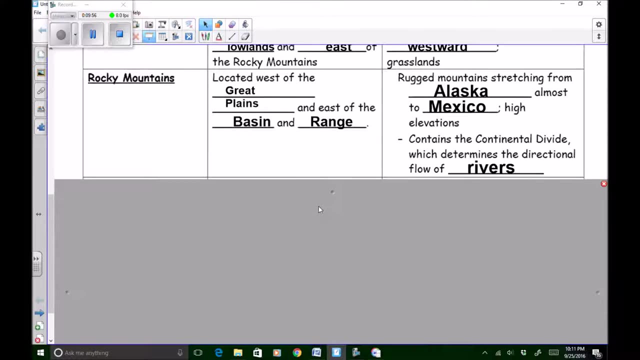 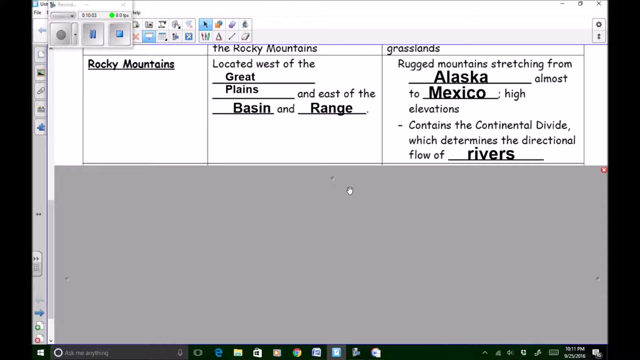 the Continental Divide, which determines the directional flow of rivers. it's called the Continental Divide, of course you know rivers flow downhill. all right again, you can pause this if you need to. I want to scroll on down to the next region. that was a Rocky Mountains located west of the Great Plains and east of the basin and range rugged mountain. 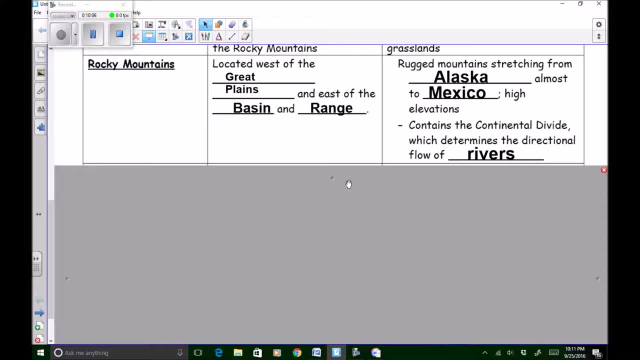 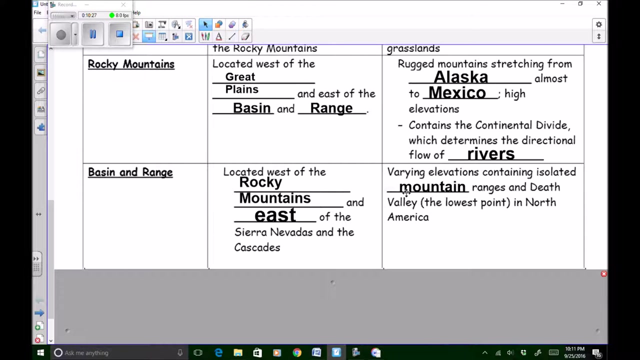 stretching from Alaska to almost to Mexico, with high elevations, and contains the Continental Divide, which determines the directional flow of the rivers. that determines which direction the rivers flow. I want to go ahead and unveil the next one here, which is called the basin and range. now, the base and range. remember, pay attention to what I'm saying to you. 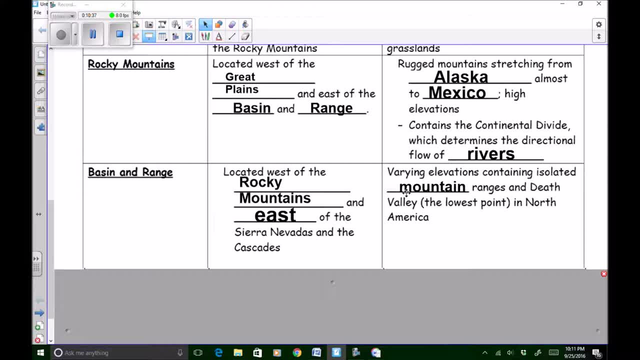 because- because I'm trying to explain what some of this stuff means- the base in range is located west of the Rocky Mountains and east of the Sierra Nevada's and the Cascades. okay, so if you go to the Rocky Mountains and you go west, you'll hit the basin and range region east of the Sierra Nevada's, west of the Rocky Mountains and located west of the Sea. 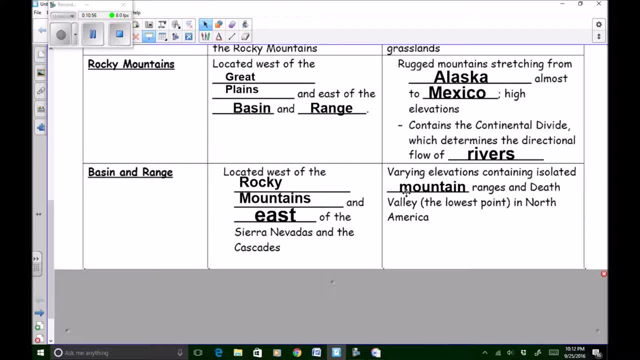 Lindsey Mountain Mountains and the partis andserian valleys will be located east of the Sea, of the Sierra Nevada's, west of the Rocky Mountains, east of the Cascades. it has varying elevations, lots of different elevations, containing isolated. now, the word isolated means that they're hard to get to, they're not next to a lot of. 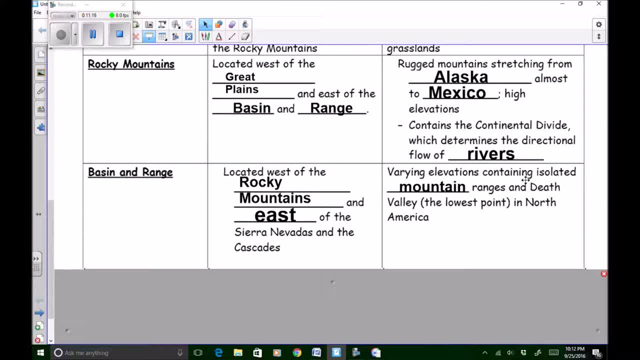 people. they're hard to get to ice, containing isolated mountain ranges, and it contains a place called Death Valley which is in California. Death Valley is the lowest point in North America. it actually gets very hot there in certain times of the year. you're talking 120 degrees sometimes, which is very hot. 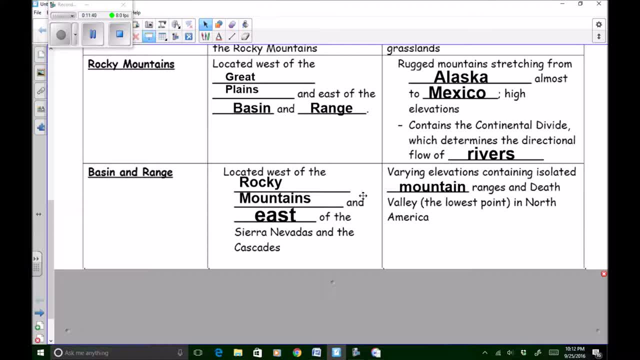 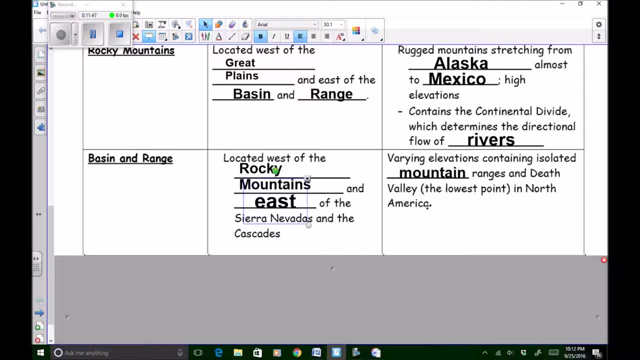 lowest point in North America. that was the base center range, again located west of the Rocky Mountains, east of the Sierra Nevada's and the Cascades. varying elevations, lots of different elevations, containing isolated mountain ranges, mountain ranges that are hard to get to. that's what isolated means, okay. 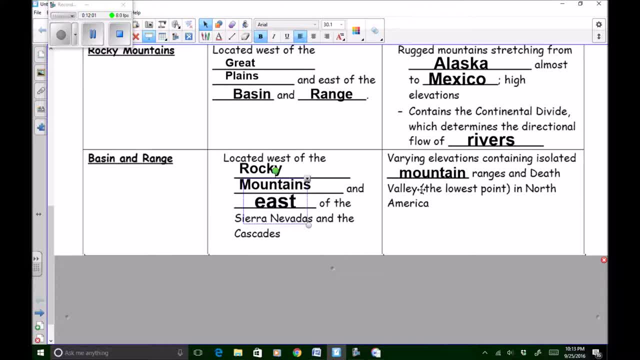 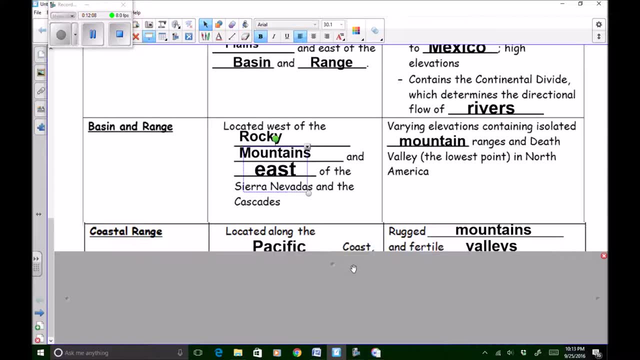 they're kind of by themselves- and Death Valley, lowest point in North America. okay, I'm gonna scroll down a little bit more to our next and final region, which is the coastal range. the coastal range is located along the Pacific Coast. now this is where you could talk to Miss Hall about this and this is basically. 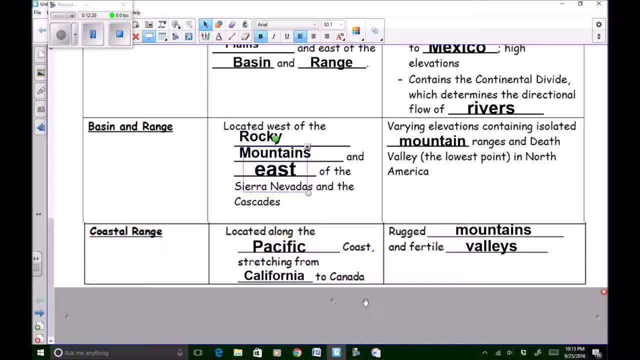 where she's from. she's from probably close to the coastal range, not maybe not right in, maybe not right in the area, but close to the coastal range because she's from Washington State, the state of Washington, which is different than the state we've been our cast, their country's capital, Washington DC. okay, it's located along the Pacific Coast and it'sorácáo a bahcanía, dimまりalar deieseo está elstra canadaさん adopción que tiene la isle live en Washington. estela return a violación przypadku de la pasión local al sur y medio deh Brahmanía Cáceres order de no sur refugio norte stylo n記得 que se encuentra en la capital de Washington DC, because she's from Washington state, the state of Washington, which has a new state of Washington which is different than this table, than our kids, their countries. 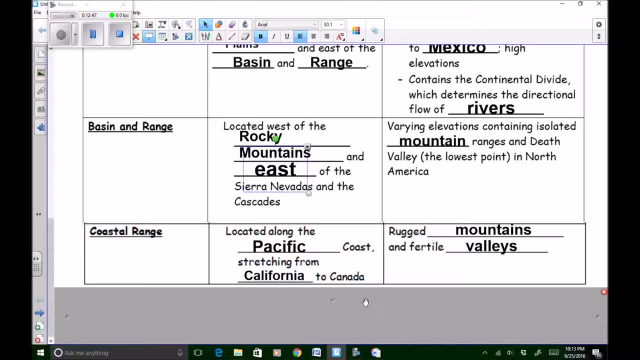 capital, Washington DC. okay, it's located along the Pacific coast, stretching from the state of California- that's where Mrs Mack is from- to Canada, all the way up to Canada, our northern neighbor. to describe this, you would say it has rugged mountains. the mountains here are again steep and hard to get around and fertile. 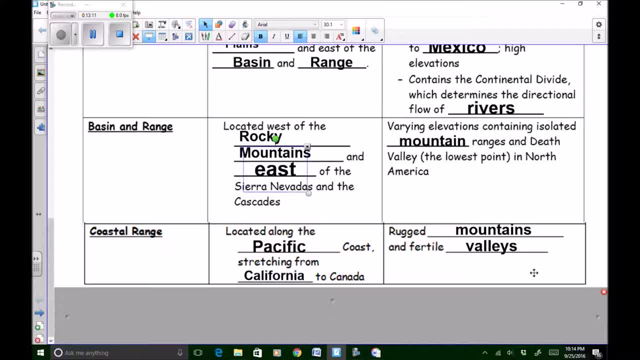 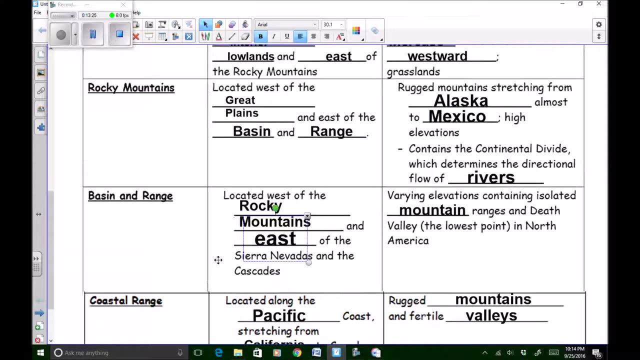 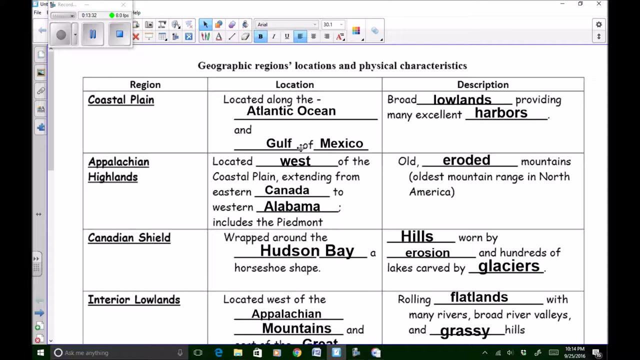 valleys. fertile valleys means that the valleys are good for growing crops. okay, that concludes our eight regions of North America's geography. the eight geographic regions I will scroll back up. go through them once again. the coastal plain located along the Atlantic Ocean and Gulf of Mexico. the Appalachian. 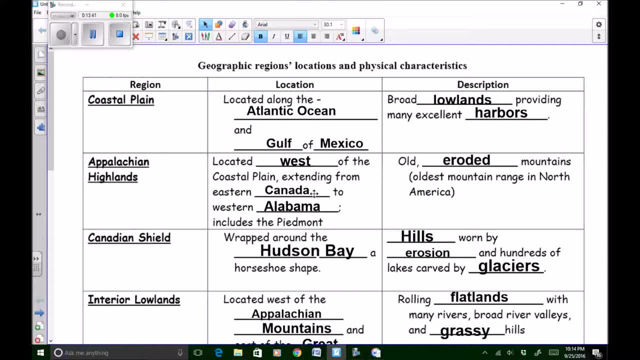 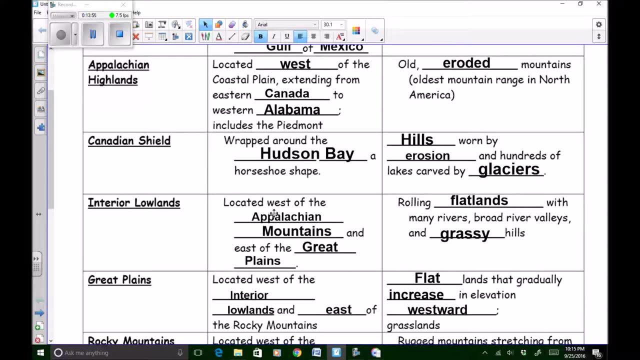 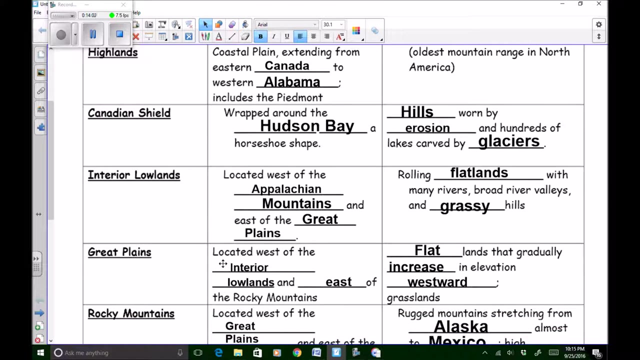 Highlands, located west of the coastal plain extending from eastern Canada to western Alabama, includes the Piedmont Canadian Shield wrapped around the Hudson Bay in a horseshoe shape. interior lowlands located west of the Appalachian Mountains and east of the Great Plains. the Great Plains, located west of the 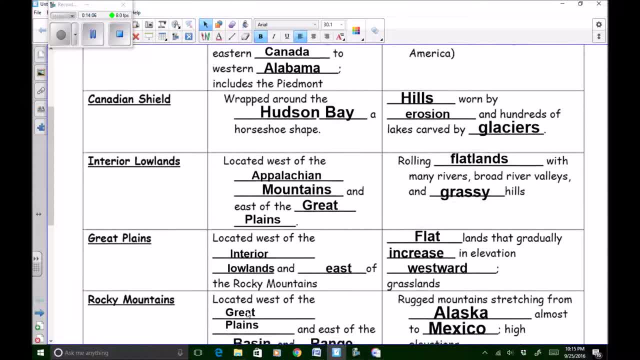 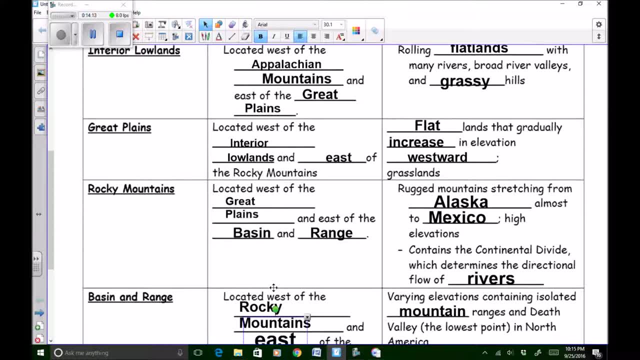 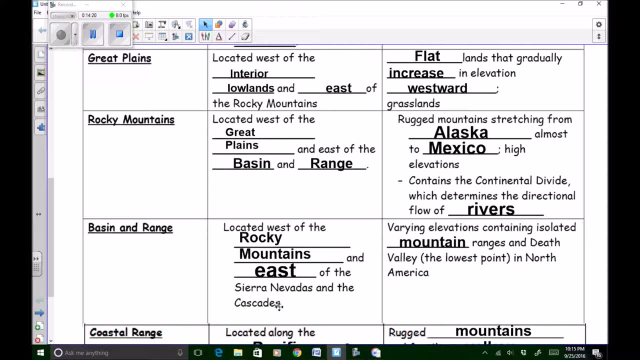 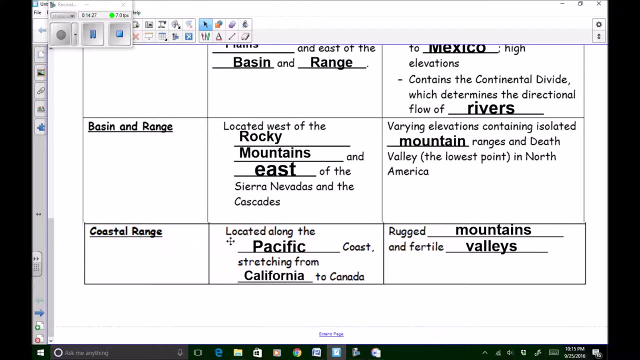 interior lowlands and east of the Rocky Mountains, Rocky Mountains located west of the Great Plains and east of the Basin and Range, then the Basin and Range located west of the Rocky Mountains and east of the Sierra Nevadas and the Cascades, and then, finally, the coastal range located along 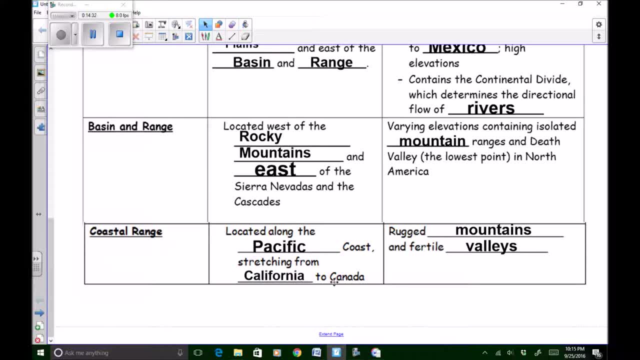 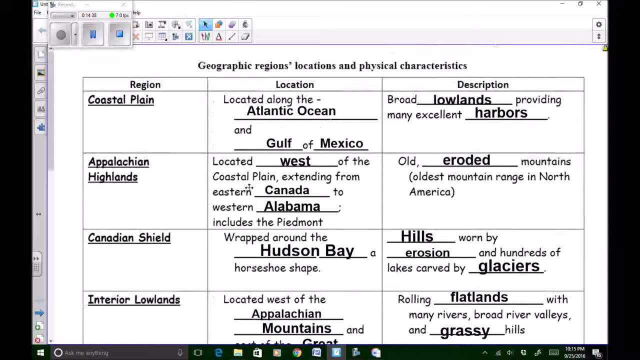 the Pacific coast stretching from California to Canada. those are eight geographic regions of North America. Please make sure you have this study guide, as well as also known as your notes page, filled out for your geographic regions of North America. Thank you.